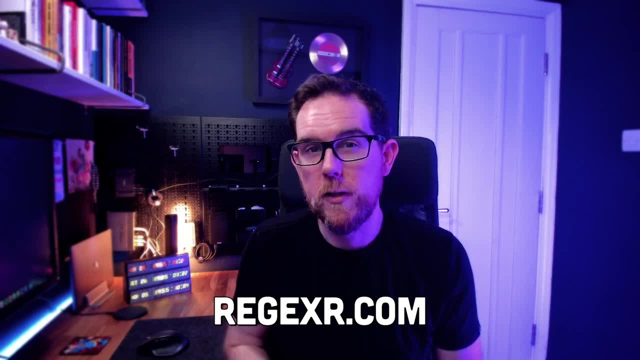 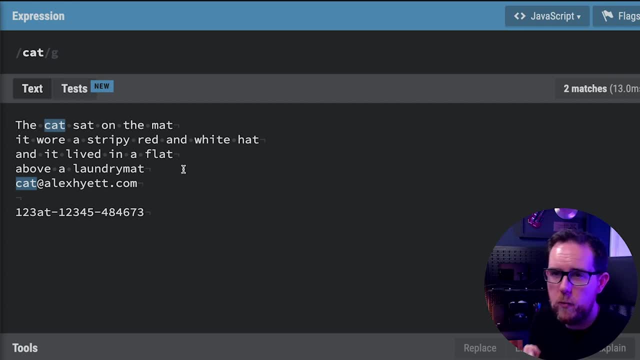 for all of my examples. I'll put a link in the description if you're interested and want to follow along. So here I've got a nice bit of text. You can see, here I'm searching for cat. You can do simple stringed searches with regex, but obviously that's not what makes it powerful. 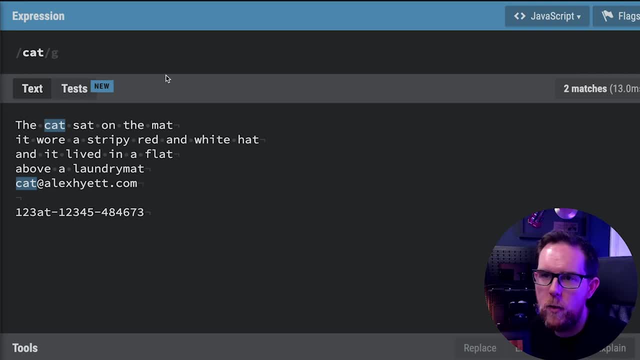 So there's a few different special characters you can use here to help you with your searches. So let's say, instead of cat we were interested in anything that starts with a letter or a number. So here there is a special character that is slash w. So with slash w it will match every. 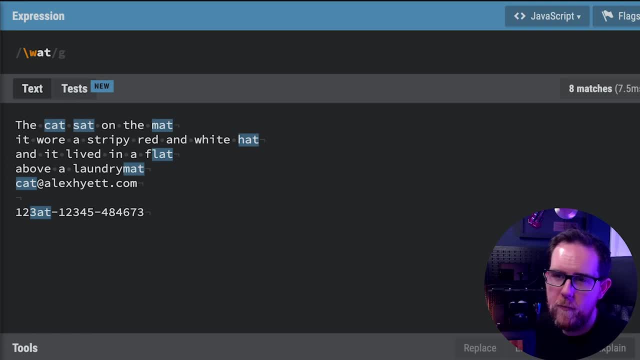 alphanumerical character as well as underscores. So here we're finding cat sat as well as things where we've got a three here as well, that's matching. You can also match just numbers with a slash d. So here we can see we've just got this three at. that's matching at the bottom. 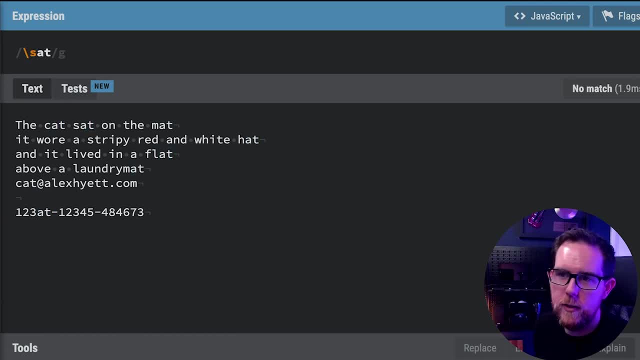 We can also match things like spaces with a slash s, So this will match spaces as well as tabs and new lines. So we haven't got anything here that starts with a space and an at, but if we get rid of the t, then this should match a few things as well. So here we can see we're matching each of. 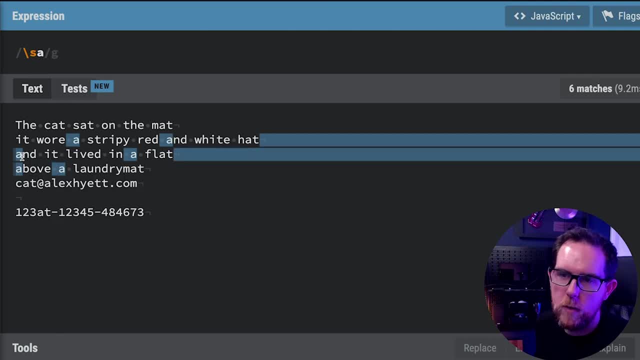 the spaces with an a, and it will also match where that a is. So we can see here that we've got a letter and a number here, and we can also match spaces with a slash d. So this will match a few things as well. So if you want to search for anything, that's not 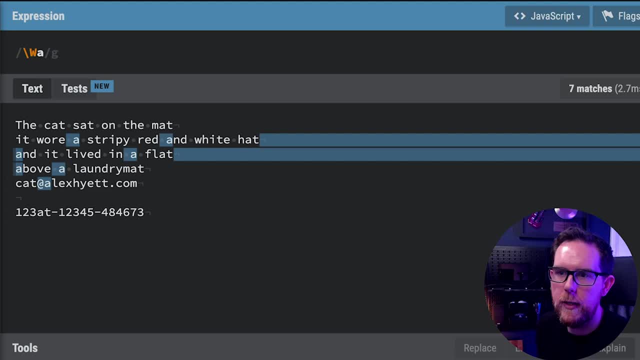 a letter or a number. you can do a capital w here, So here we can see it's matching just the spaces. or we can do not a space with a capital s, Or we can do not a number with a capital d. You can see here that that at here with a number isn't matching. There's also another special. 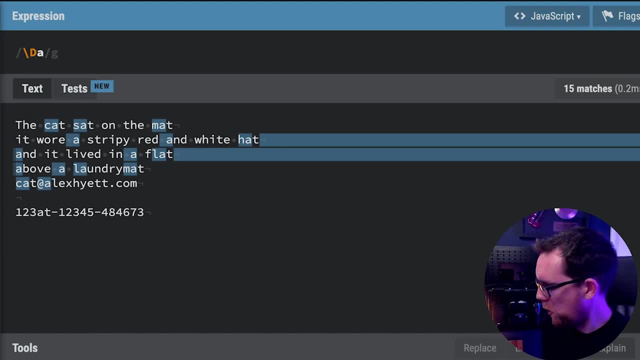 character in regex that's used to match any character in your string and that is a dot. we add a dot in. we can see we're matching everything apart from new lines here. now, obviously this is matching where we only have one character followed by a dot, but say: you don't care how many. 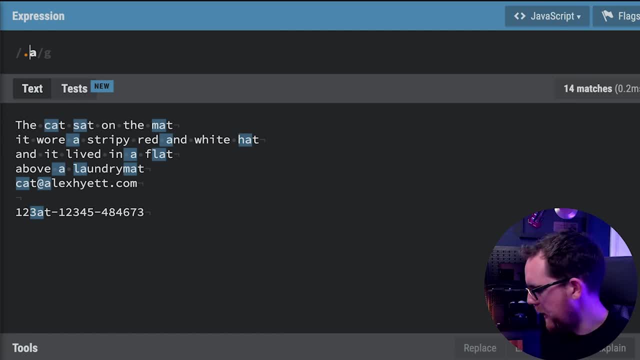 characters you have beforehand. you just want everything ending in an a. so here we can do a dot star, which matches zero or more characters. there's also a plus, which matches at least one character. so you can see, here it's very similar, but it's matching at least one. and we also have 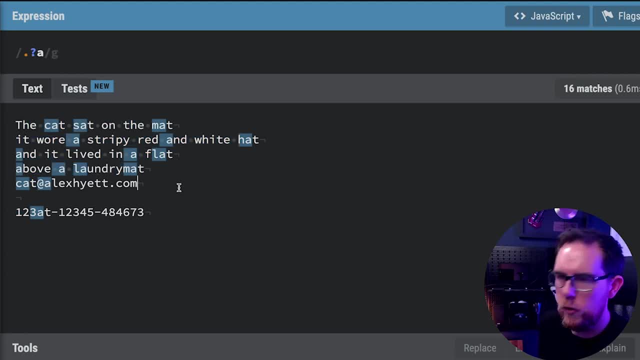 a question mark, which means it's optional. so if we had a on a new line, it would also match that as well. now let's say you wanted to match when you had exactly three a's. so here we can see we're matching three a's because we've got this dot question mark here. but if we wanted to match 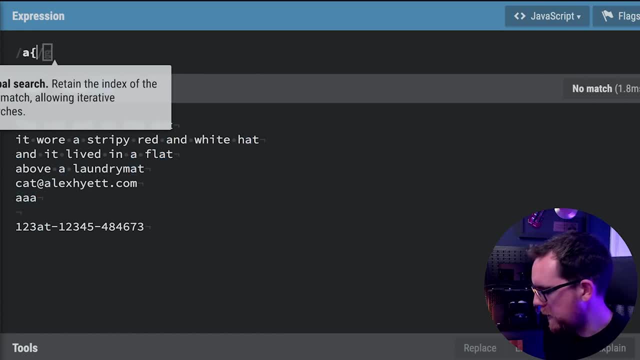 exactly three a's. we can use a curly brace in here which matches only when there's three occurrences of an a if we add in a few more a's in here. so we've got another four here and then another five. if you wanted to match all of these, then you can also do a comma five which will give 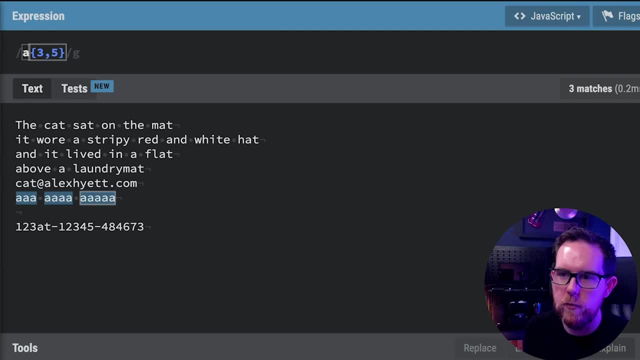 you a range to match everything where there's an a in the range from three to five of them. in regex it's also possible to put in a range of characters to match for. so if we change this back to at, we can see here we're matching on cat sat mat but say we only wanted to match it if it starts with: 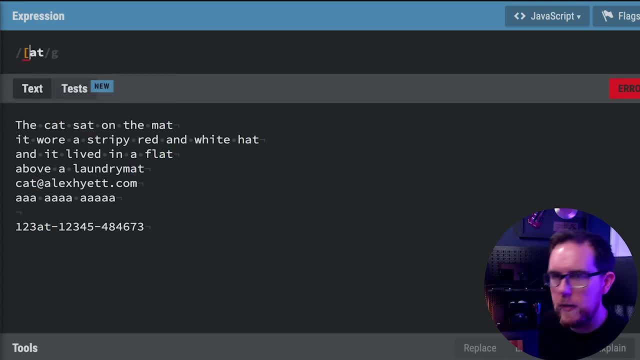 a, c or an s. here we can put in square brackets this time put in c and s and then close bracket and you can see, here we're just matching on those occurrences. you can also include ranges as well. say, we only want to match from things that. 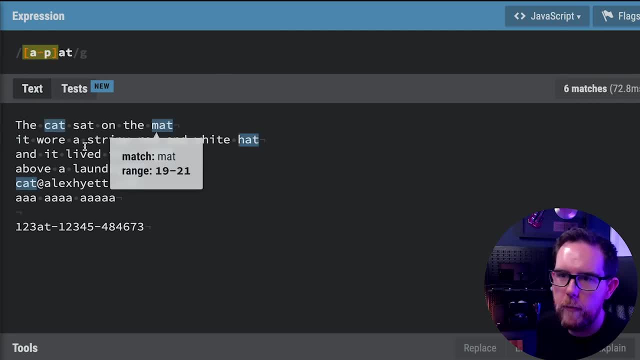 range from letters a to p. you can see here they're also matching cat mat, but we're not matching on sat. you can also do the negative of these groups as well, so say we don't want to match anything that's a to p, we can put a hat symbol on there, and when, therefore, we only match. 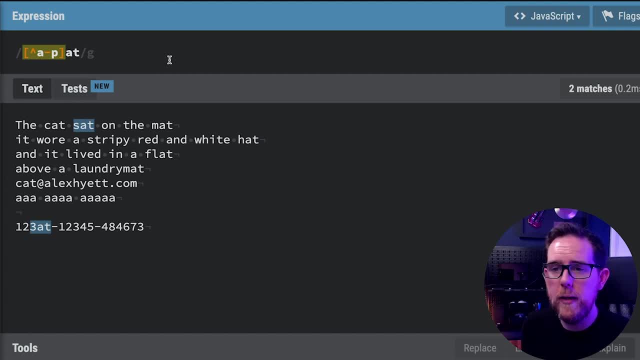 on everything that's not in a to p. so all of these are really useful for finding particular patterns in a string. but what if you want to extract some of that information and use it in your program? so let's say, we're interested in email addresses, but we only want the domain. 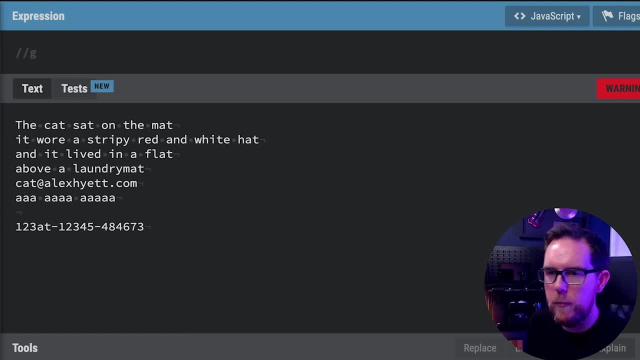 of those email addresses. so in this case i'm just going to do a slash w to find everything before my at symbol. now you might want to have a look on google and find a regular expression for email addresses that caters for every single type of email address. so we want any number of these. so 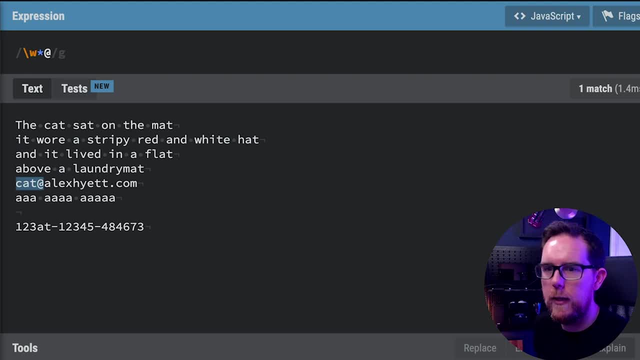 this is where we put a star in. and then we want an at symbol to say it has an at. then we're going to do another slash w for us with a star to say: give us everything after the at symbol. and then we're going to do a dot. now, in this case we could put a dot and it will match. but we actually want 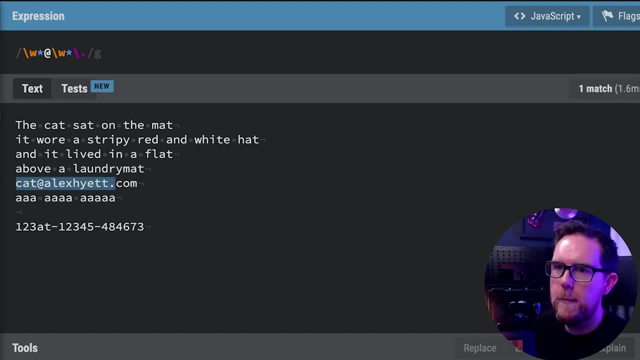 a dot. so we need to escape it with a backslash. and then we do another slash, w, to end in our dot com with a star. so here you can see it's matched that email address nicely. now to get the domain of that email address we need to add in a capture group. so to do this we add in brackets. 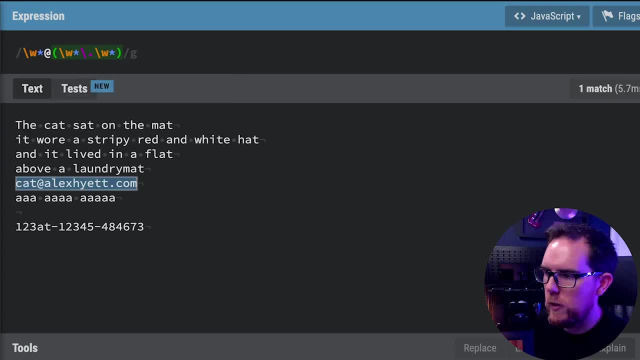 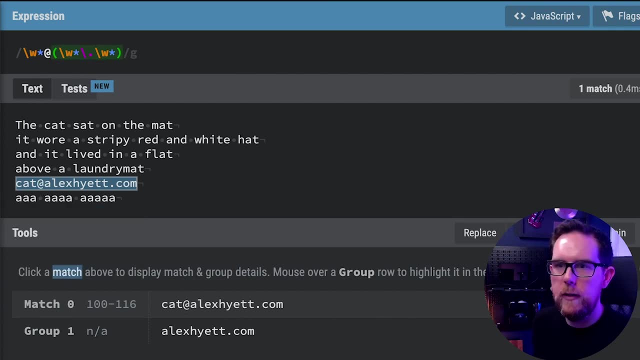 around the bit that we're interested in and you can see here it's still matching. but if we go to details on here we can see that we have a new group and the group matches our domain name. now you can add multiple groups. so let's say we want to add a group to our email address and we can. 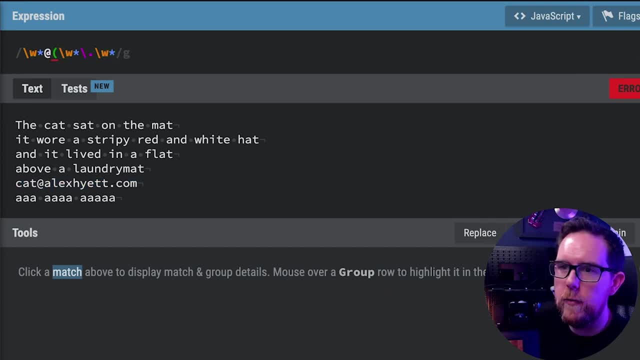 say, we're going to split out the domain extension from the domain, so we can do a bracket here and then another one after the dot to match that as well. so here you can see, we now have two groups: one for the name of the domain and the other one for the extension. so this is great for things like 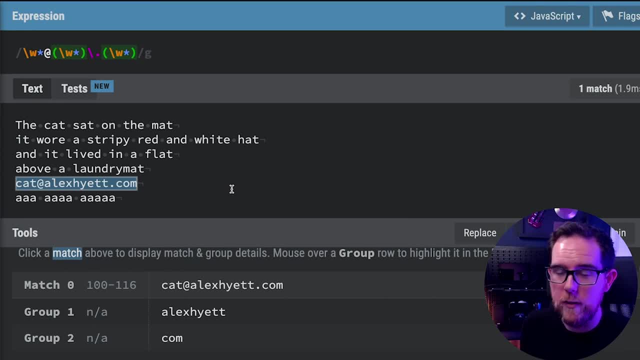 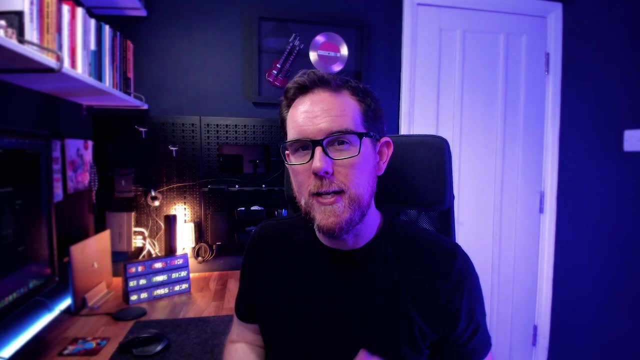 file names. if you need to match a load of file names but you want to extract what the extension is, you can do that with regular expressions. now, one of the aspects of regular expressions that people find particularly confusing is positive and negative, look aheads and look behinds. 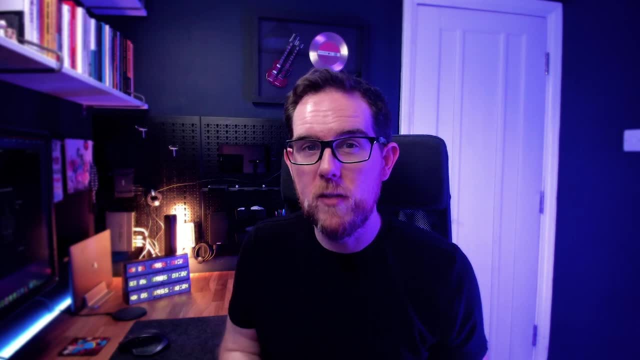 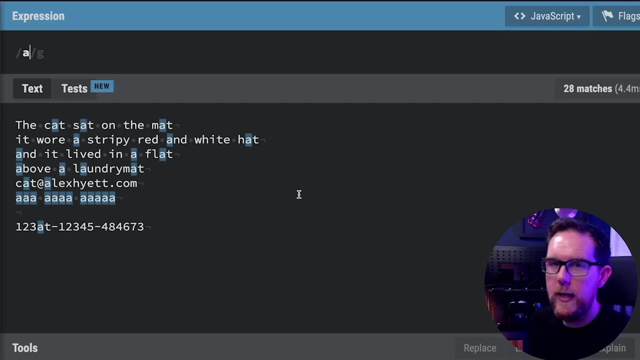 they're not actually that hard whenever you want to match something that is preceded by something else or has something else after it. that's when you use these positive and negative look aheads. so let's have a look at an example. so here we're matching on every single a but say: you only want. 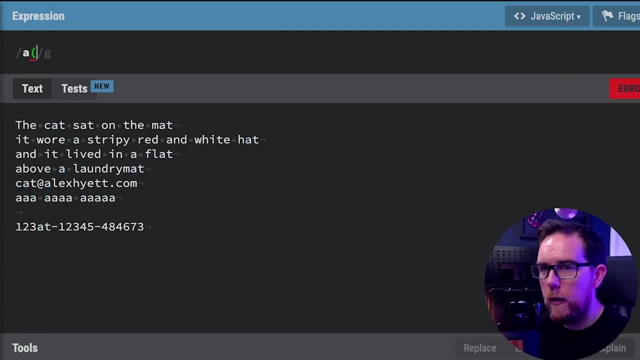 an a if it's followed by a t. here you can put in a bracket followed by a question mark and then equal t, and that gives us a positive look ahead. so you can see now we're only matching the a's where it has a t after it. but let's say we want the opposite. we only want a's where it's not. 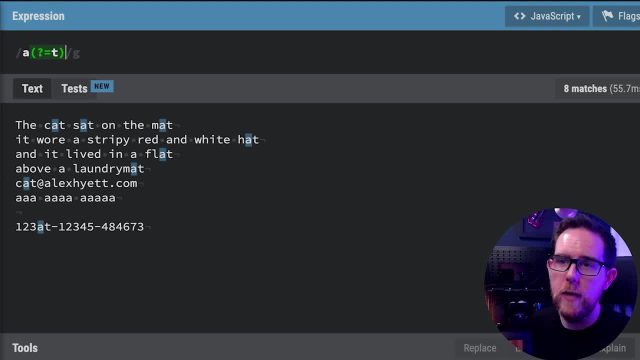 followed by a t. this is what we call a negative look ahead. so we're going to add a negative look and to do that, we just replace that equal sign with an exclamation mark, and that will give us all of the occurrences where they have an a that isn't followed by a t: the positive and negative. 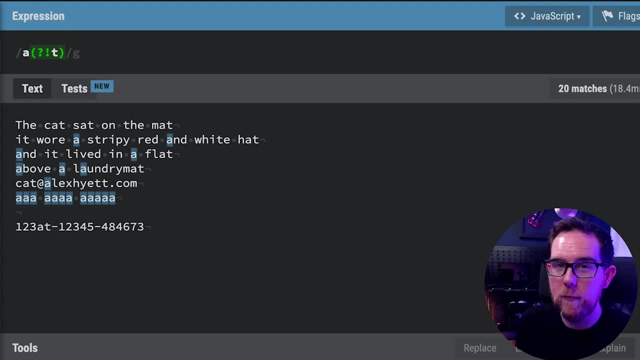 look, behinds are exactly the same, but instead we're just looking backwards instead of forwards. so here we want to see all of the a's that are preceded by a space or a new line character. so let's do this. we do open bracket question mark again, but this time we need to add in an arrow. 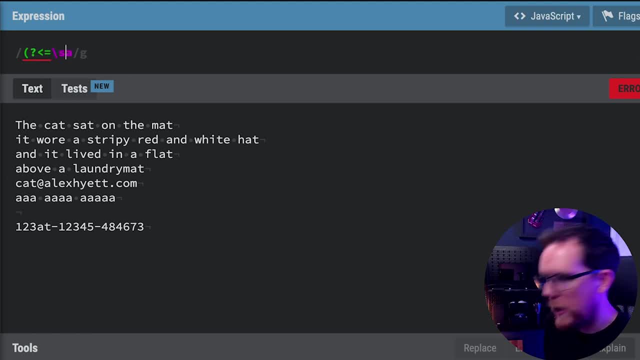 to say we're looking backwards, and then equals, and then we'll do our slash s for our new line character. so you can see, here again we've got a's highlighted, so we've got an a here because there's a space before it. we've got another a here because it's the start of a.